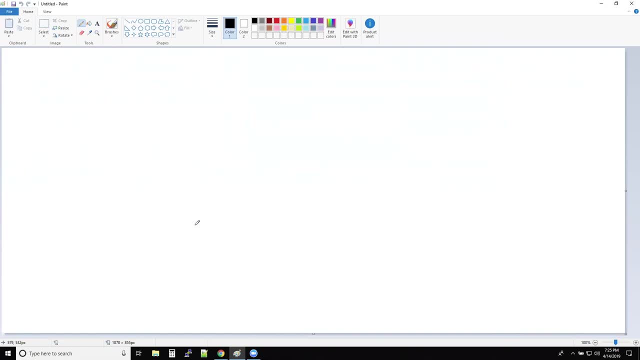 query run slow. So let us start with our first question. What do you think What might make a query run slow? Data increase: No index, Okay, Okay, Maybe statistics are not accurate. Okay, Long run- sorry, Simon, I said long run. or query insert or update: Okay, 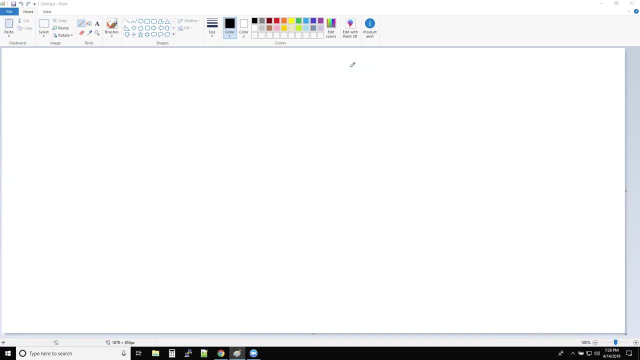 Come on, guys, think out of the box and just don't limit your thinking to things in the database. Too many users at the same time. Locks and deadlocks- Great For application design or tables that are not properly normalized: Perfect Great. 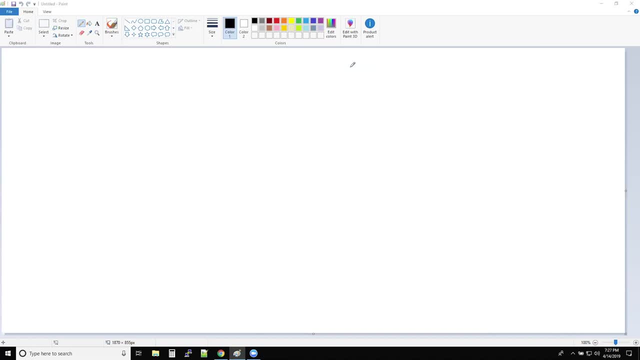 And I'm just trying to understand some more examples from you guys. What might be the other issues that might cause a database to run the queries very slow? Some kind of table joints- Okay. Inefficient IO utilization- Okay, Great. You all guys are going great. 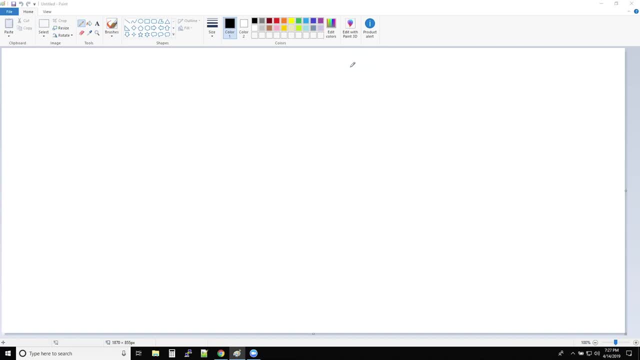 So still continue. I mean, if you have more ideas, continue. The edge condition: Great And wrong commas, Wrong commas. Yeah, I don't know, I don't know, I don't know. Okay, I don't know. 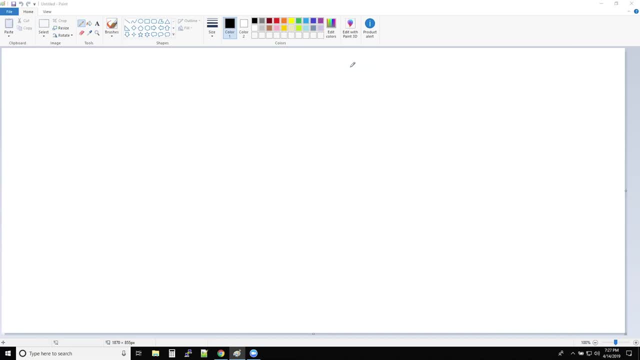 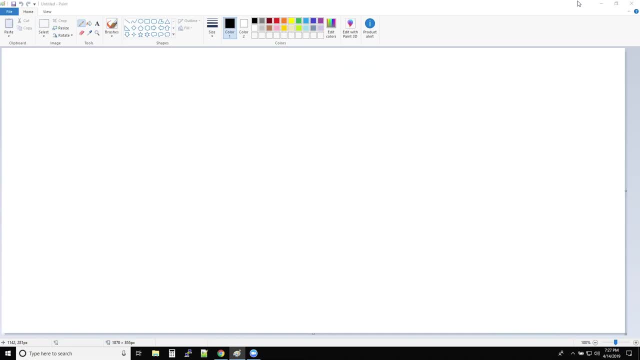 Okay, But our question is: when you hit enter, the query is running and running, and running and running, but not giving any output. So what could cause the query to run? let's take a query taking five minutes today and tomorrow it's taking 55 minutes. 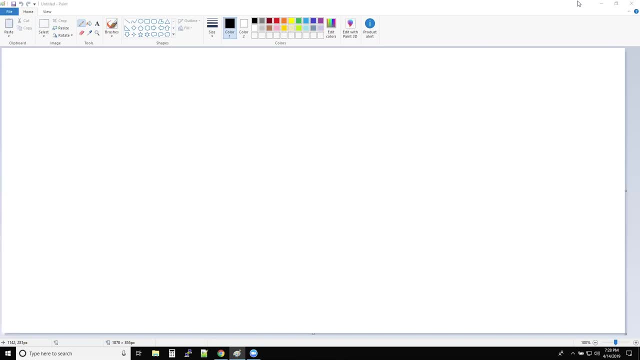 So that's a problem? right, There should be a problem. I'm there, That's it, Perfect, That's it, That dick space. It could also be from the SGA that some of their parameters They are not properly sized. 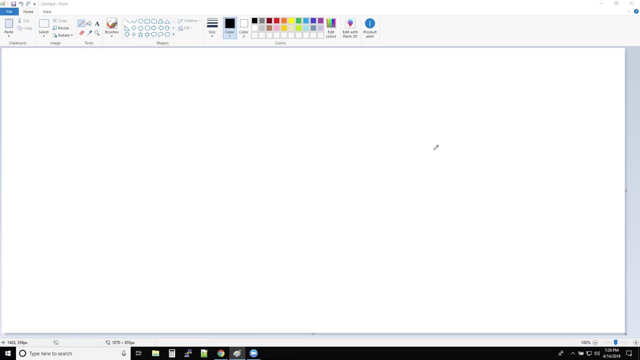 correct, great and I think, Right, right, amazing. next Columns and joints: A hot, hot passes: Okay, Mm-hmm, Mm-hmm, Okay, If someone really significant Stats are not gathered is still Right, okay. database: the buffer service: query buffers: Okay. 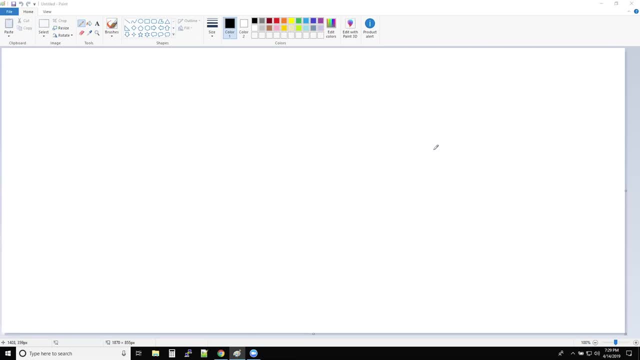 So most of the examples that you gave like I would accept, but some of them were vague and not at all related to performance tuning and You will understand it slowly because I'll be walking you through How. Okay, first we'll define how or what exactly is performance tuning? then I should, or I will, walk you through the performance tuning. 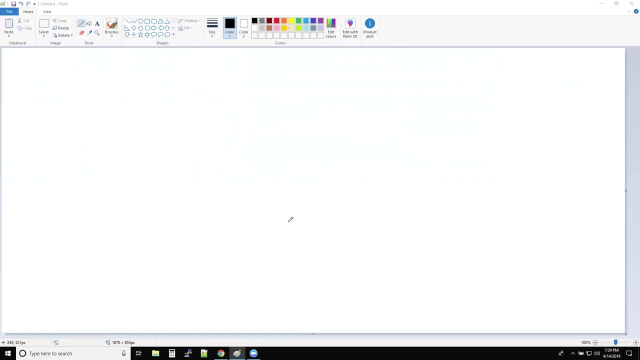 steps, like in a technical or a real world, how performance tuning is done and What is the iterative process. So, guys, at the core of performance tuning is you need to understand there are only two goals in performance tuning. There is no third or fourth goal. Okay, Now there might be some books or 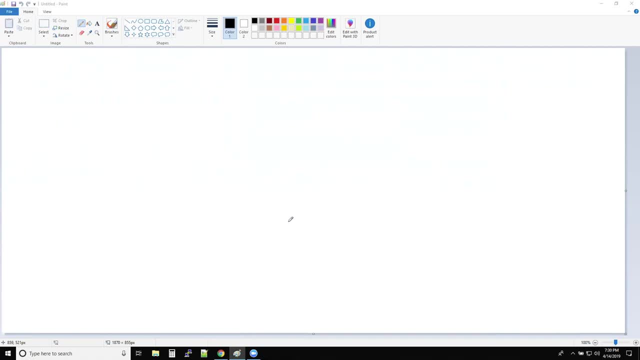 blogs that will misguide you. but there are only two goals and if you are a great DBA and if you know how to work or Fix those two goals, then you know the entire performance tuning. I'm kind of like simplifying things for you, for all of you, because 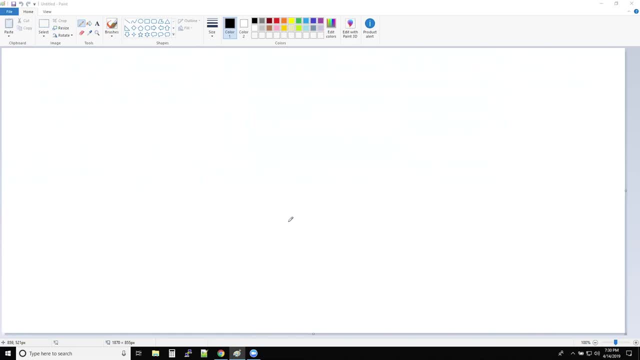 Because in this session definitely we can't look at the entire performance tuning. So The performance tuning goal that we have is there are only two performance tuning goals: It is to reduce the response time and to improve the throughput. This is something like might be some new terms for you, but I'll come come to this in some time. 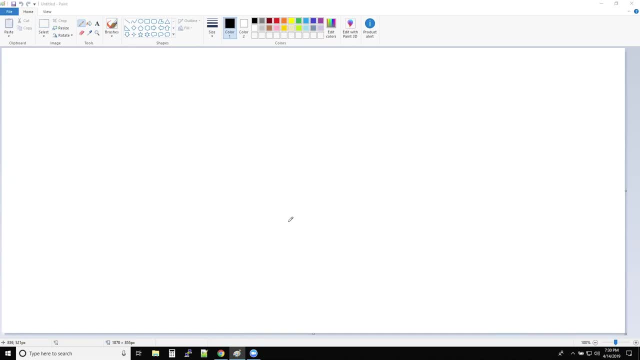 So, guys, why did we look at database locks before performance tuning? The reason was for you to understand: Whenever there is a performance issue or a query is running slow, it is not always to do with the performance tuning. there might be issue with the database locks, or 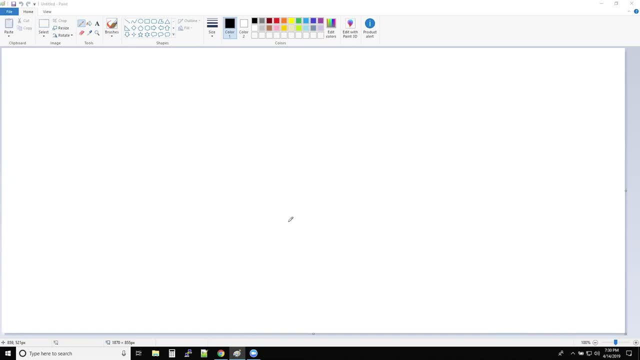 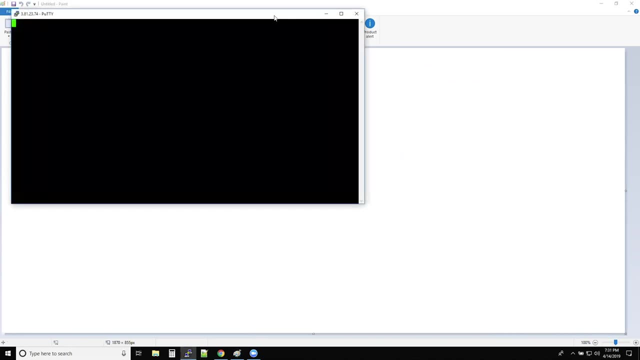 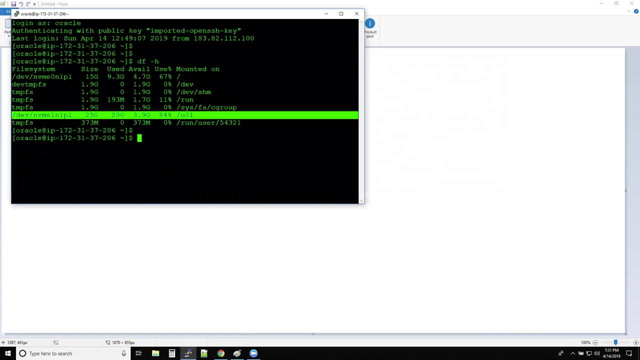 There might be issue with discus hundred percent full, So I'll show you one example. So sometimes what happens is: So we have more ten minutes to go, all right. sometimes Your disk, where your Oracle home is installed, it is 100% full. So Whenever a user is complaining that my query is taking more time. 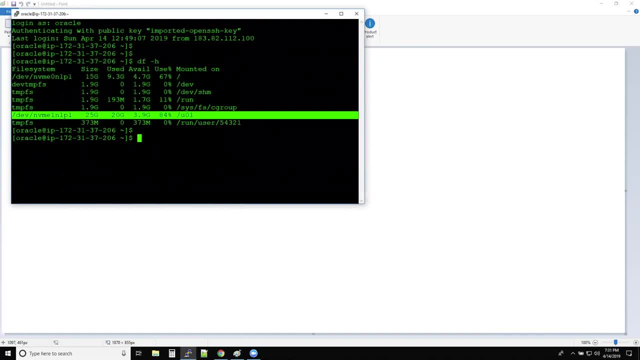 Don't right away, start your performance tuning Activity or don't write away. jump into generative and looking at the performance statistics. There might be some other issues also, okay, and so what you need to do is, whenever a user is complaining, you need to debug it in a way. 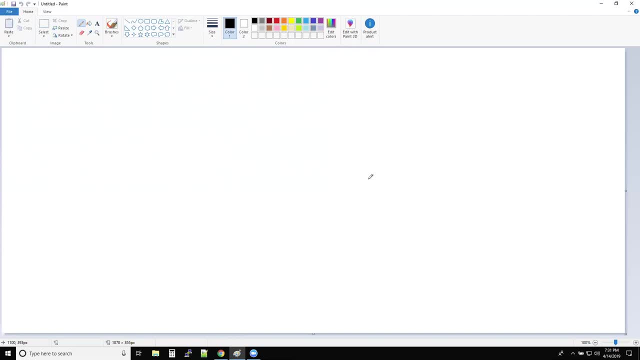 that makes sense to you because, see, a user might tell like, hey, every day my query runs uh smoothly, but today it's taking more time. at this stage you need to make sure you are asking the time difference, like how much time your query takes generally, and they might say: like it takes. 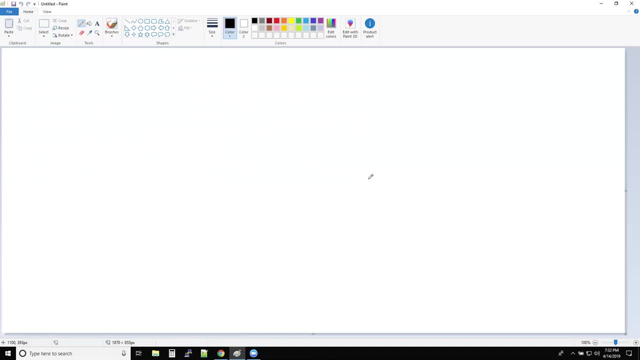 two minutes and today how much time is it taking to run? and they might say four minutes. what you can do is you can look at your database and see whether some activities were going on. was there any data load that was going on inside the database that caused heavy usage of database instance and? 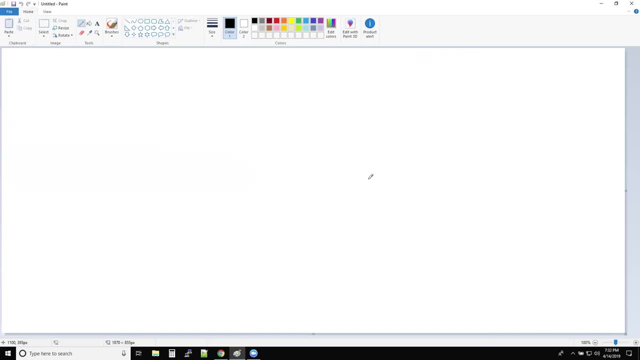 that definitely will have a small impact on the queries. so for the performance tuning, the biggest problem right now in front of dbas is that people just complain but they don't know, like how much time the query used to take earlier or what is the performance benchmark. 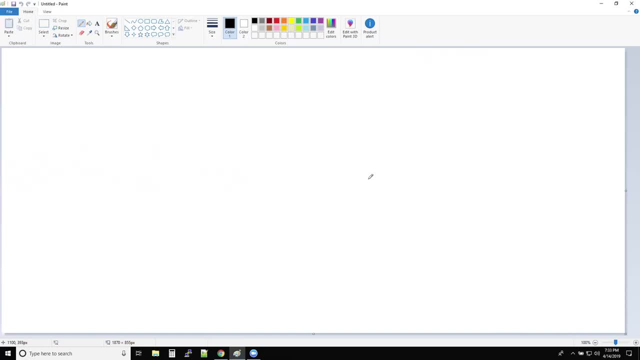 i think that's the correct term. so what happens is like: uh for in a in a banking sector? uh, definitely you cannot have one minute wait time for your clients. technically, these days one minute is huge, so you can't even have like 10 seconds of wait time for the customers. 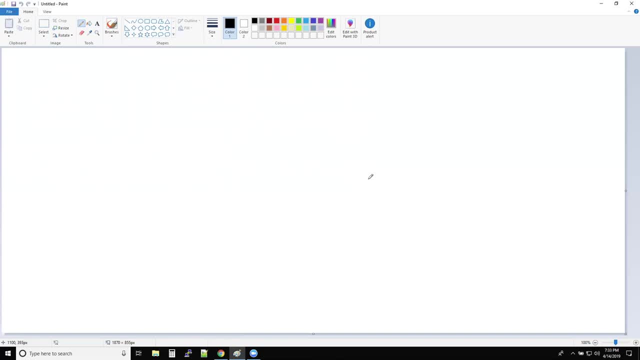 so these all are like performance benchmarks. so what happens is, when you work with clients, you define some performance benchmarks. okay, every sql that runs inside the database, or any sql that is querying a table, it should not exceed the time range between five to 10 seconds. So that way it makes your life easy as a DBA. Okay. 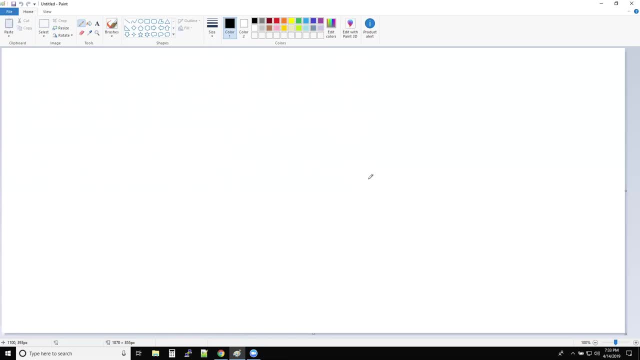 there is a benchmark and any query that's taking above 10 seconds, that means we are failing to deliver the SLA, And that's when what happens is, as a DBA, you need to tune the SQL. So before you directly jump into the performance tuning activities, don't try to take out all the 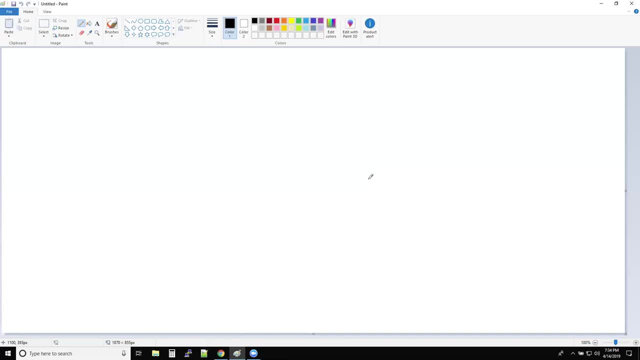 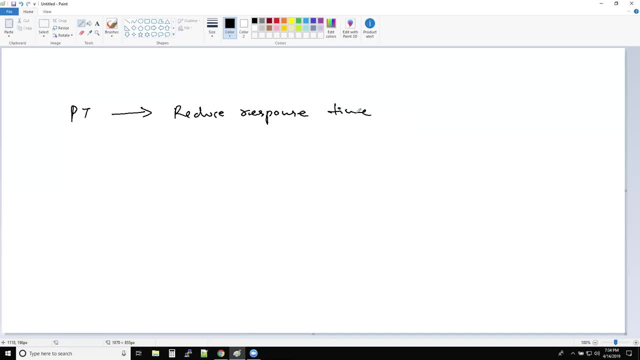 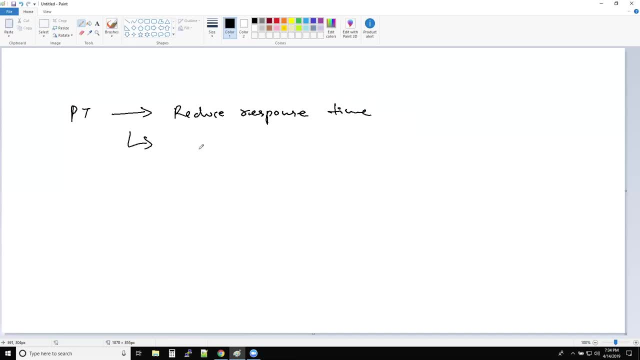 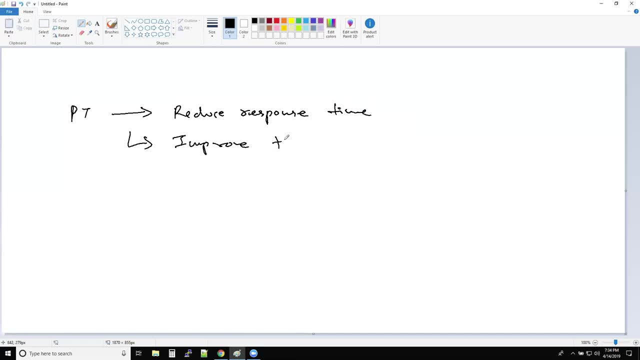 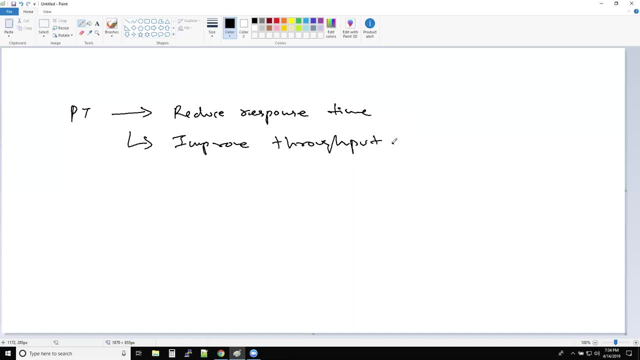 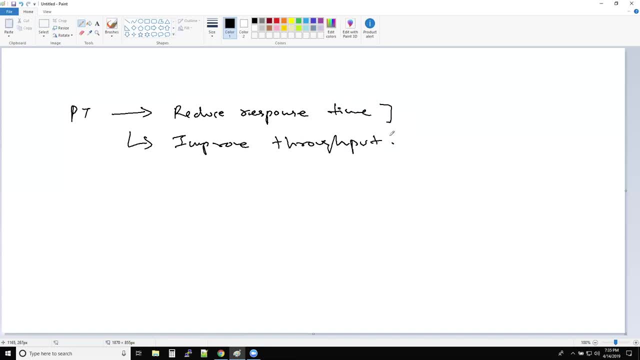 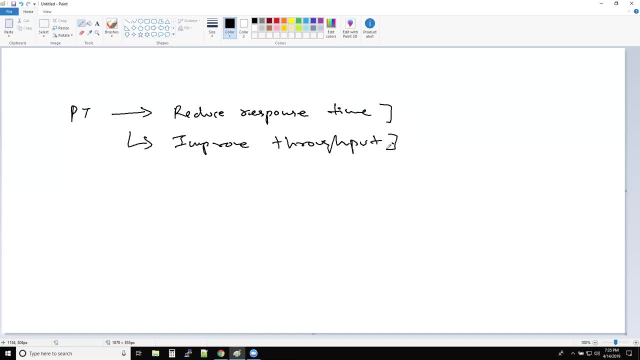 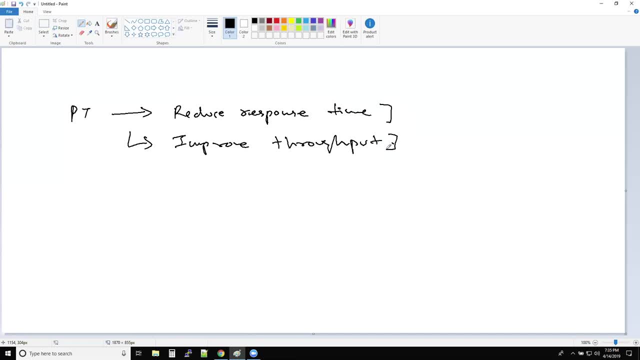 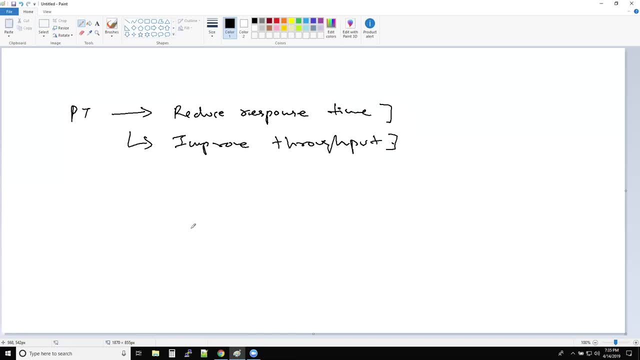 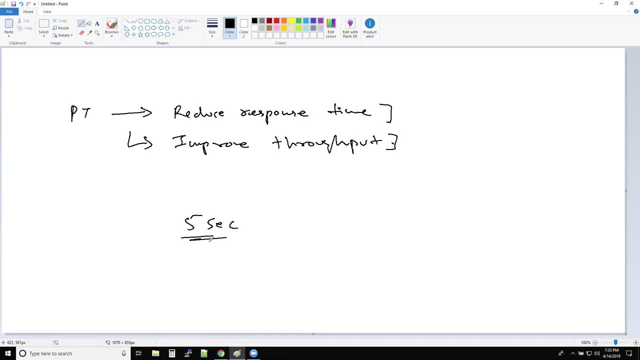 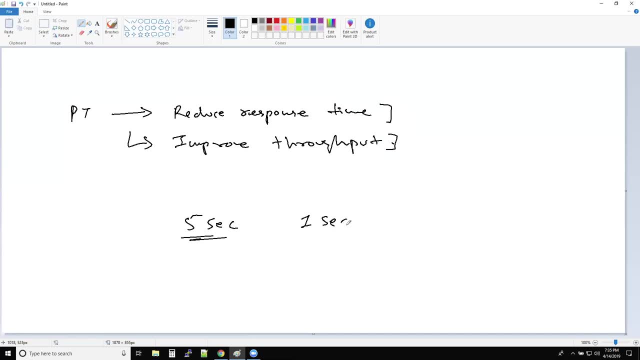 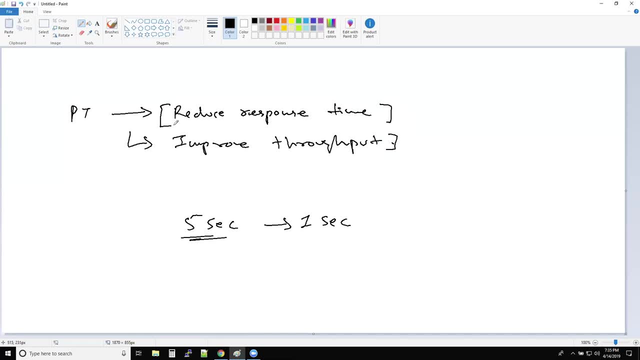 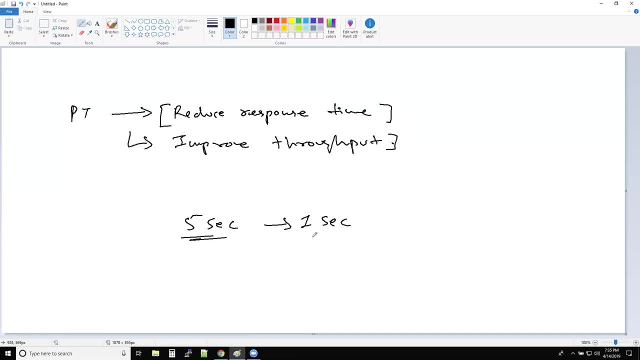 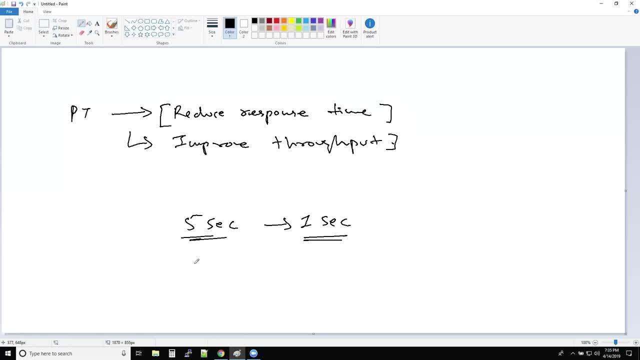 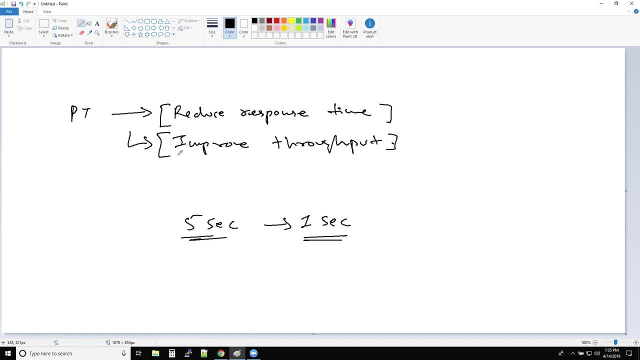 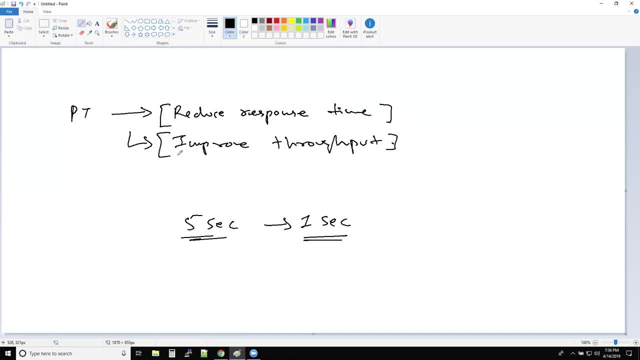 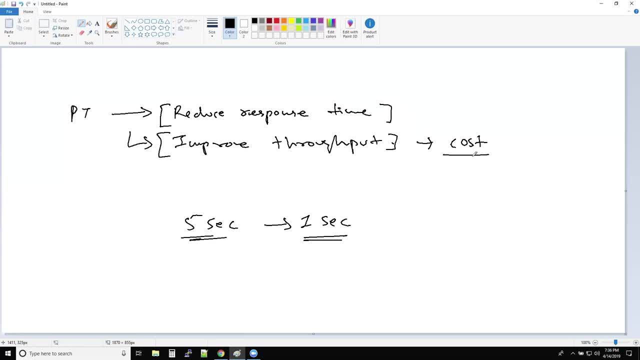 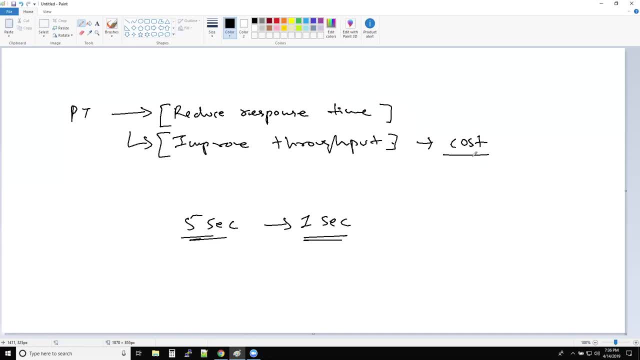 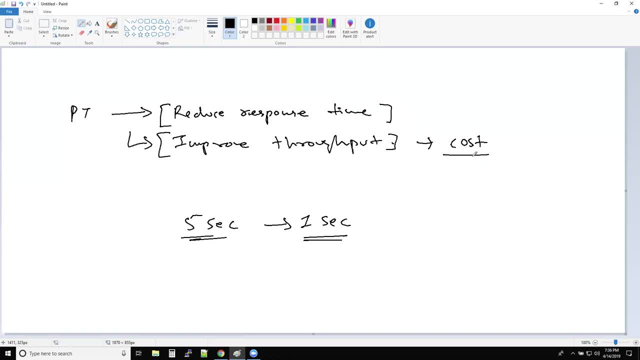 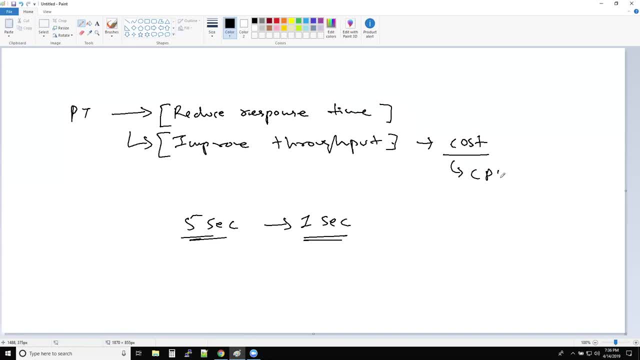 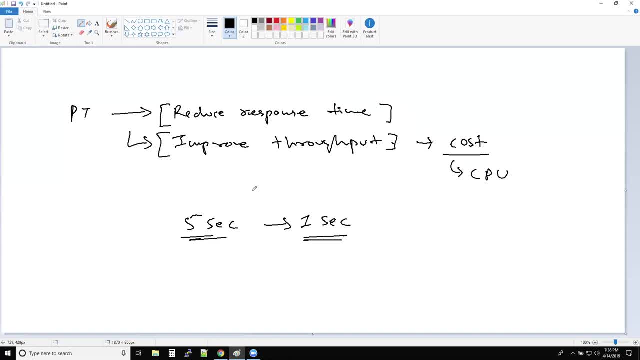 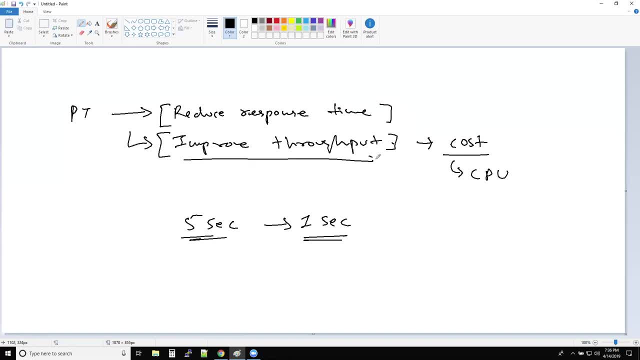 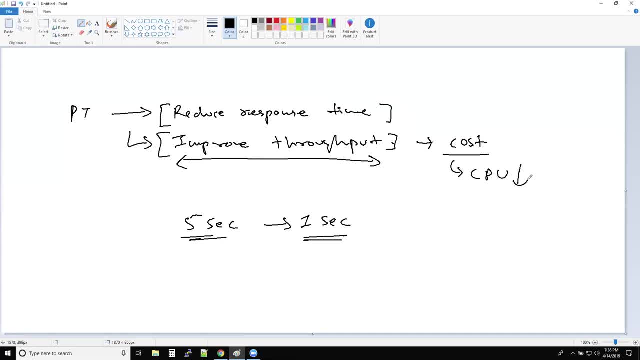 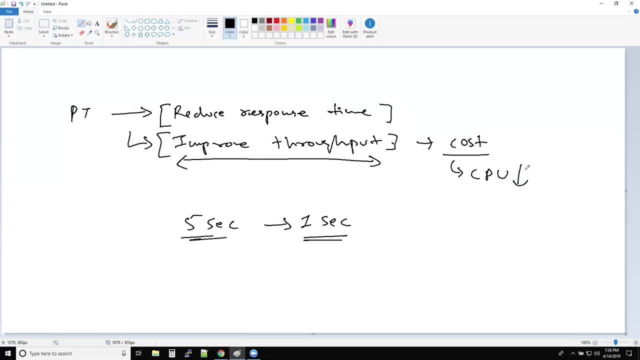 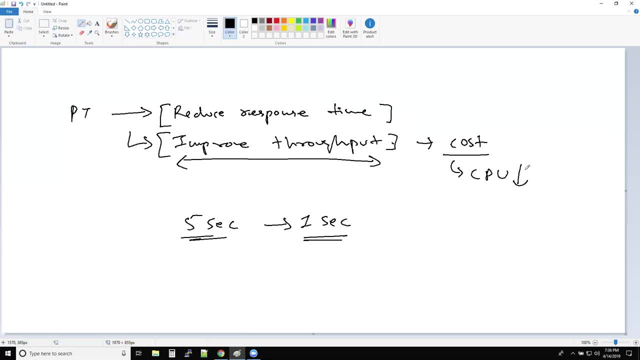 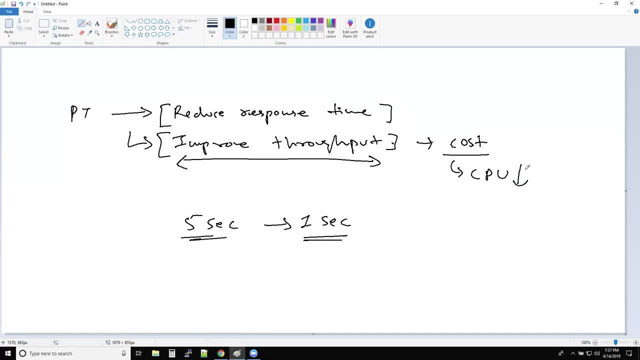 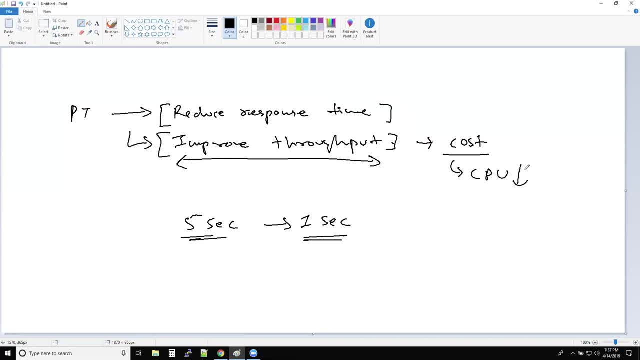 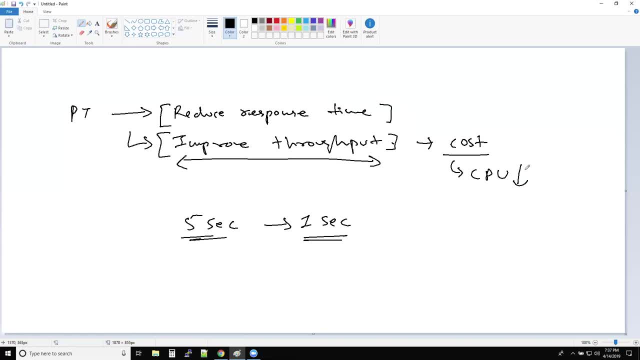 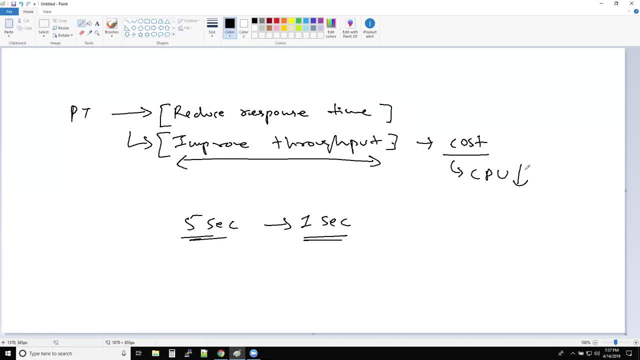 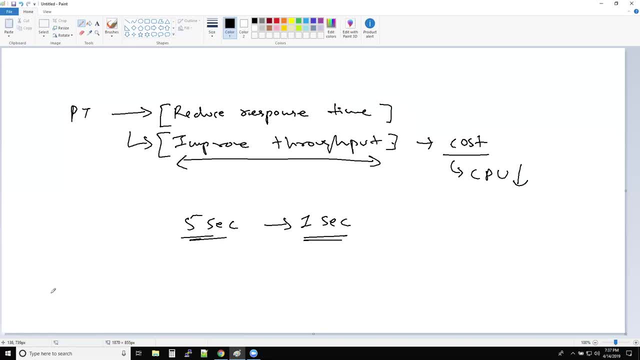 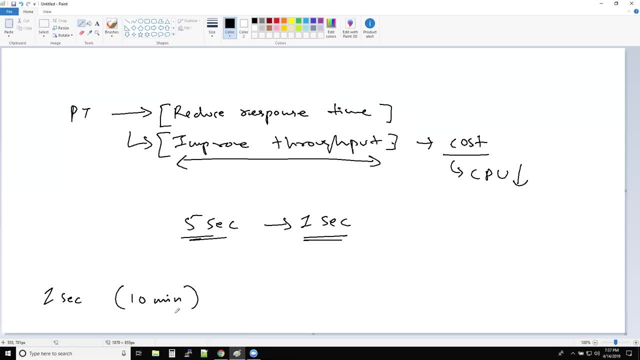 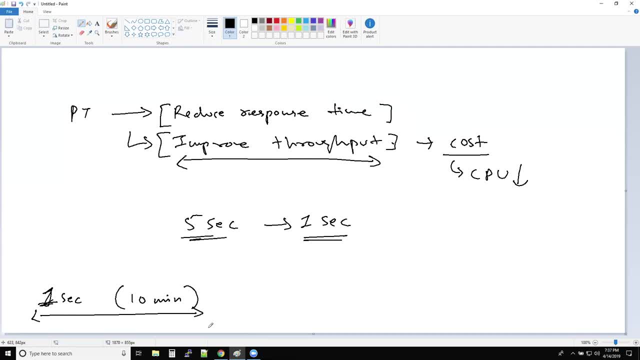 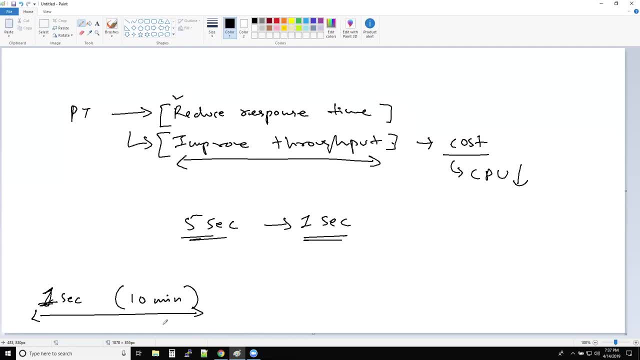 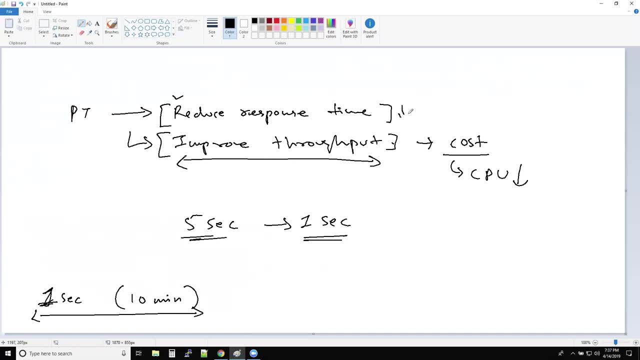 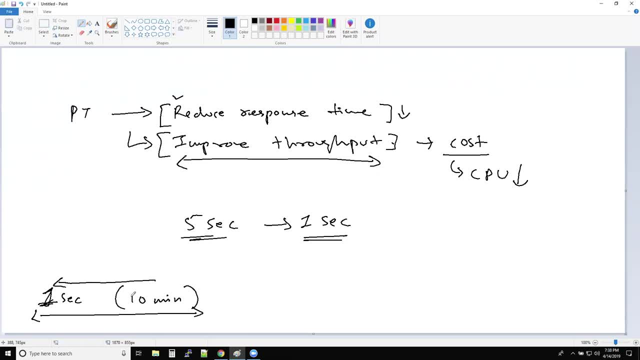 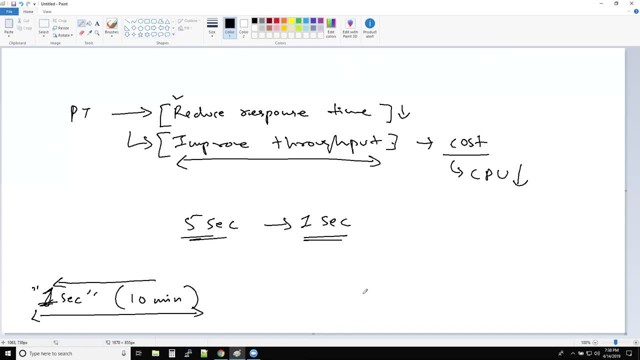 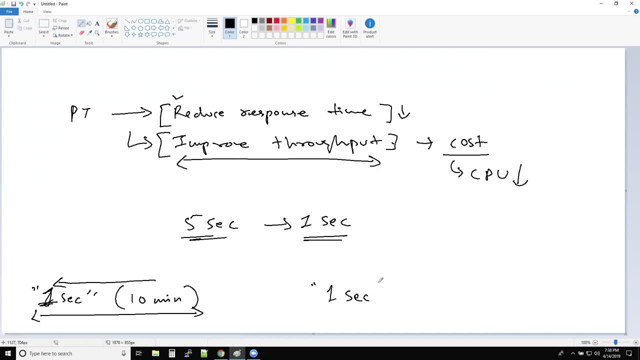 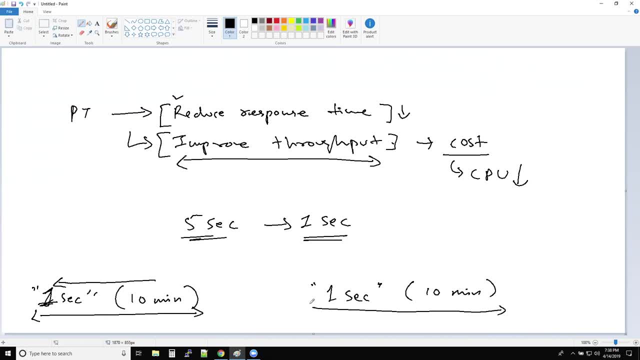 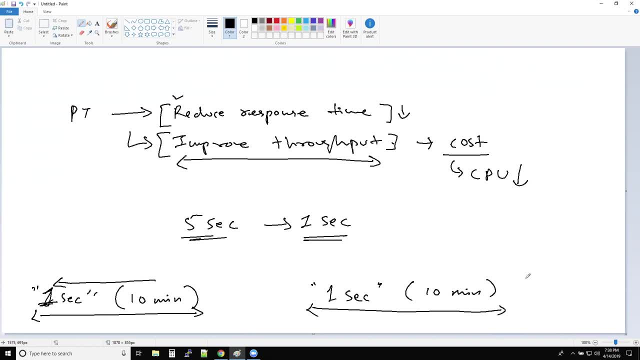 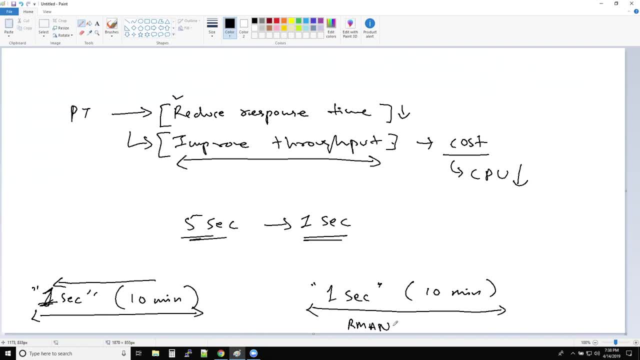 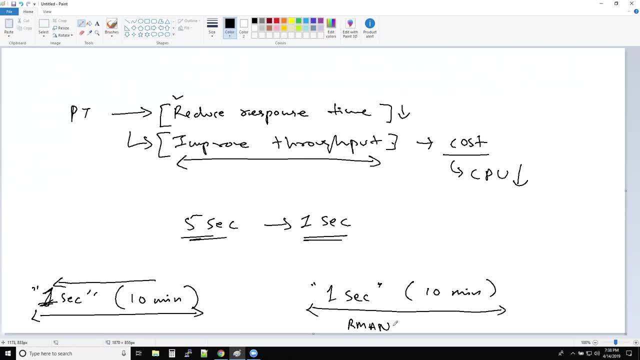 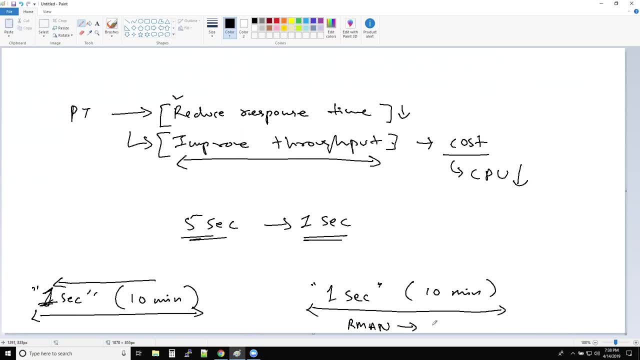 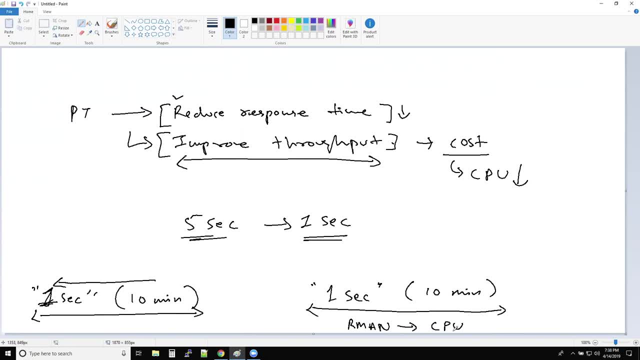 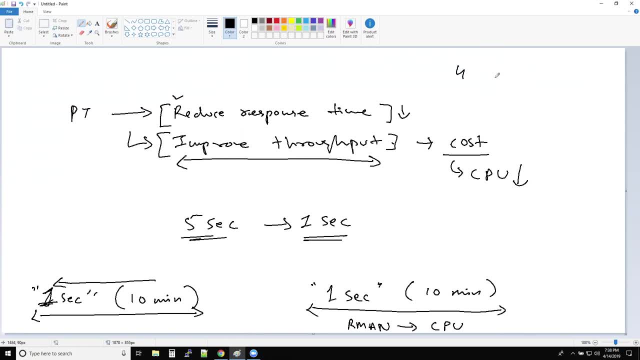 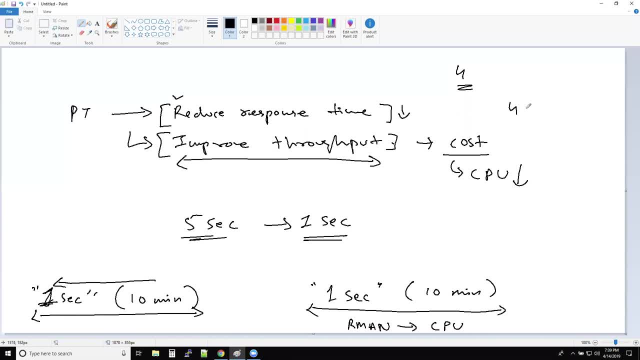 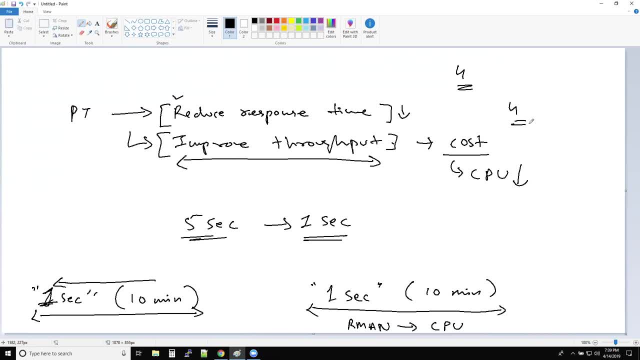 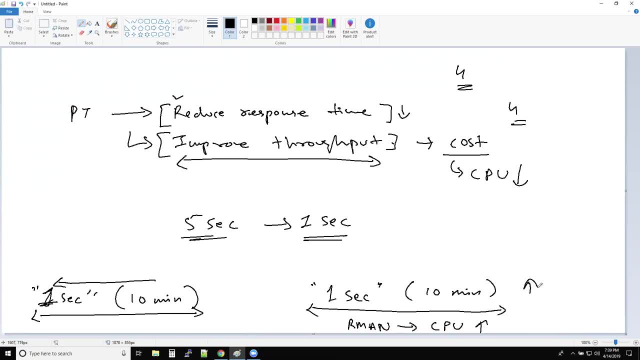 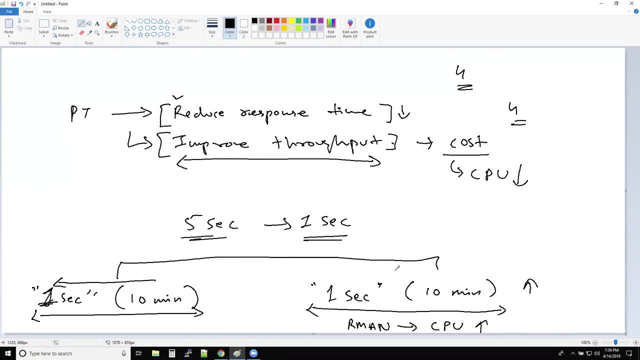 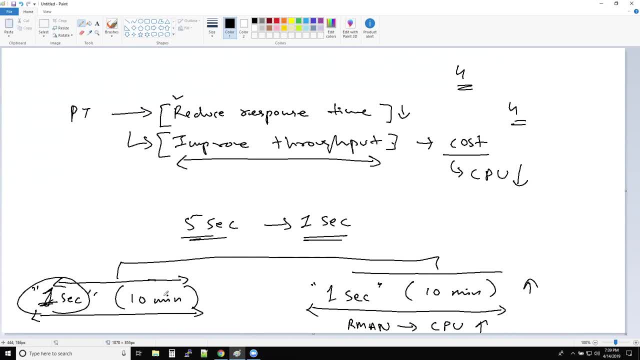 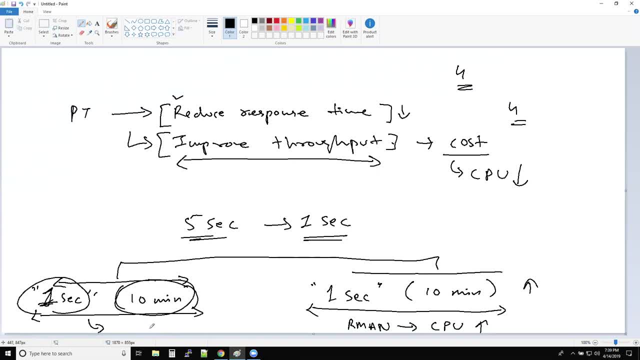 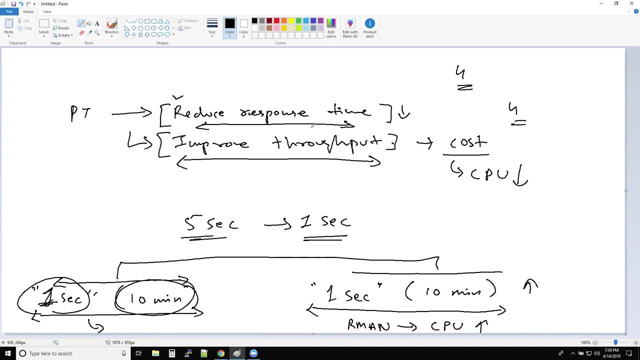 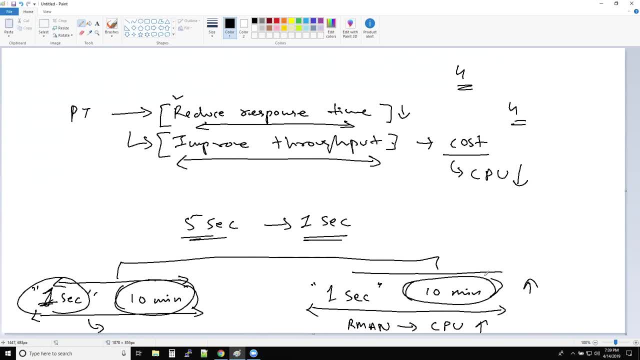 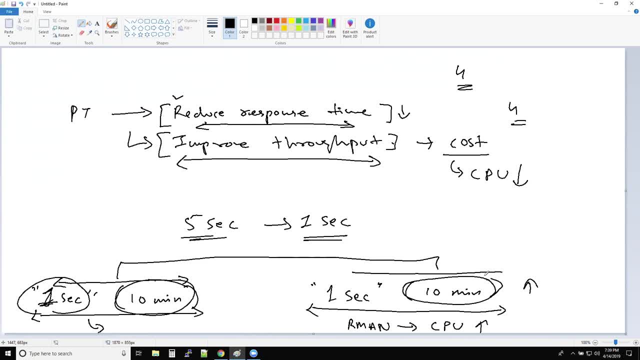 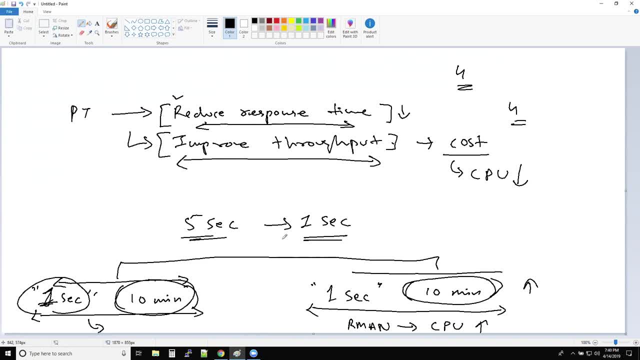 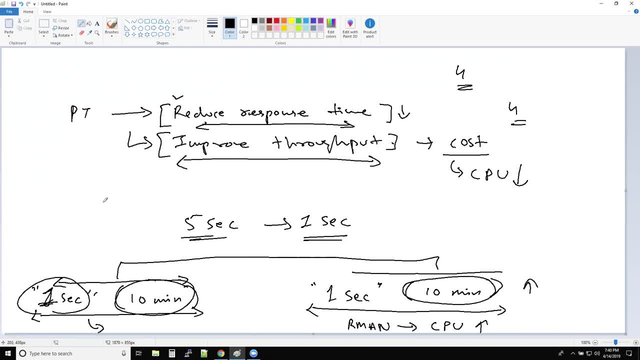 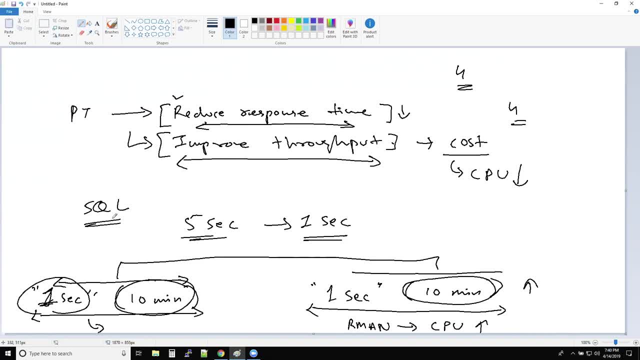 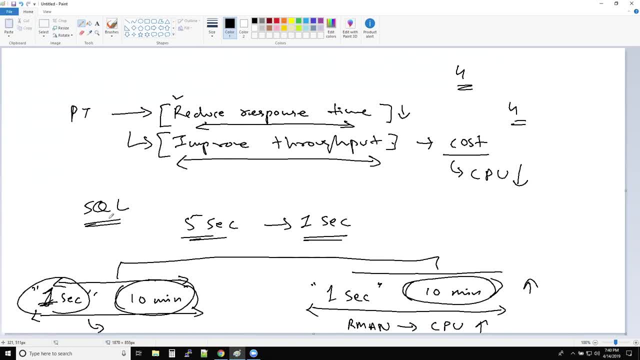 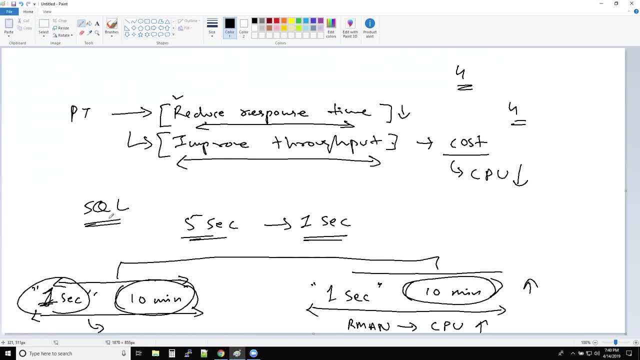 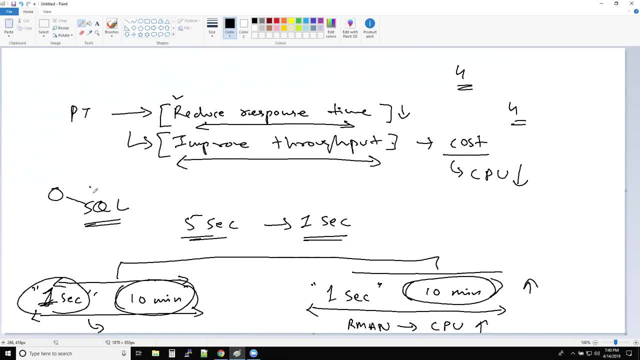 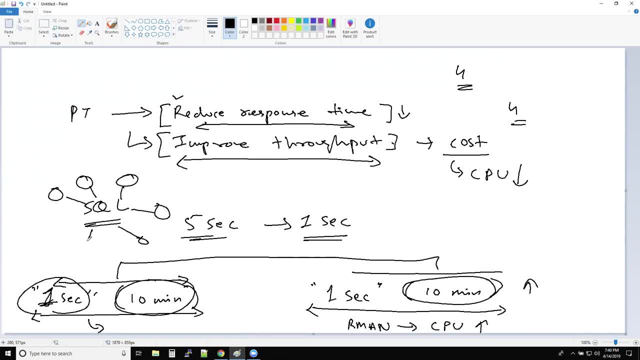 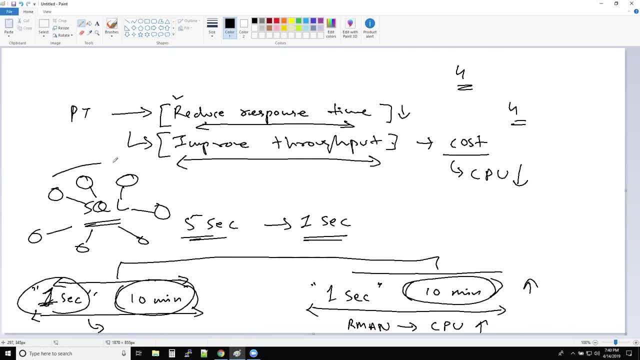 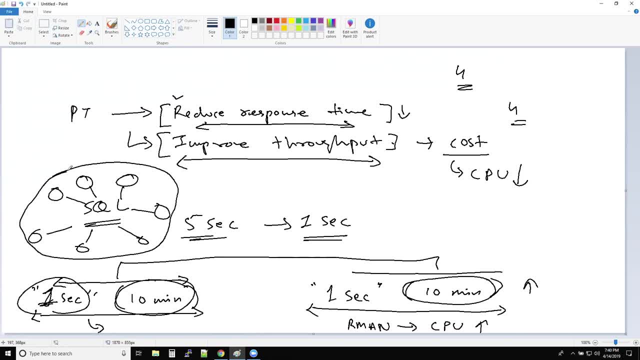 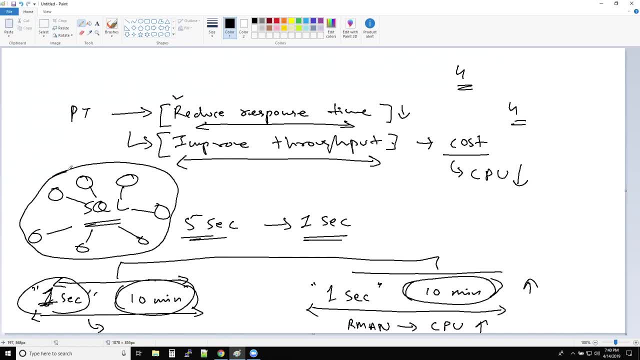 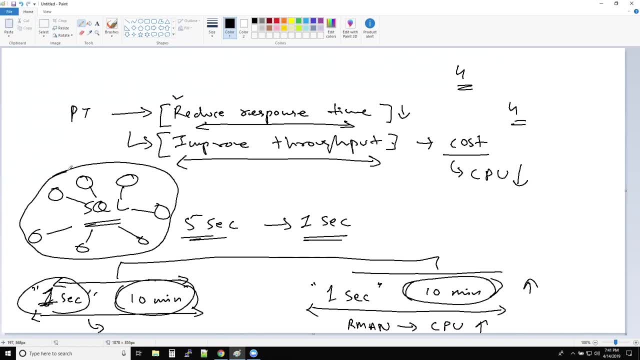 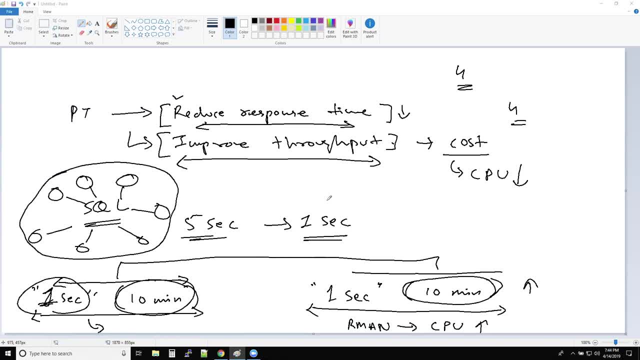 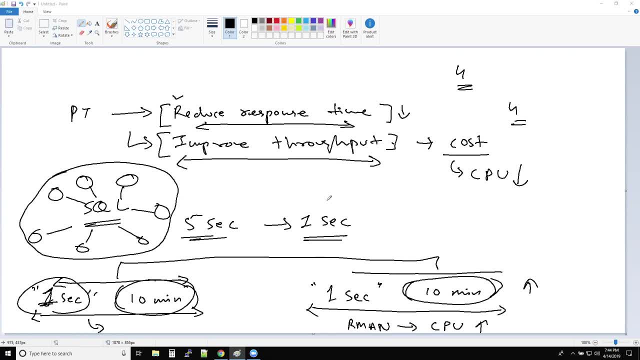 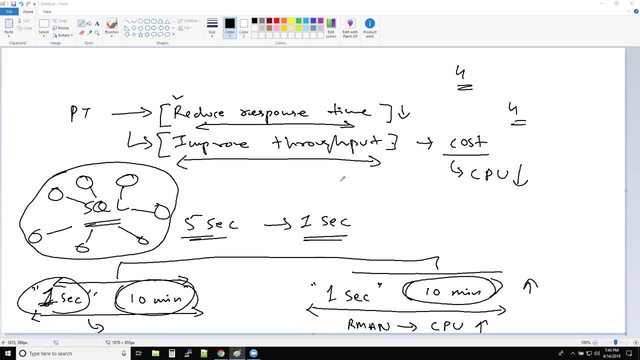 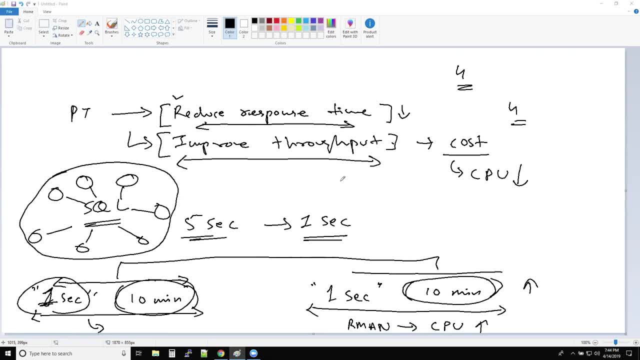 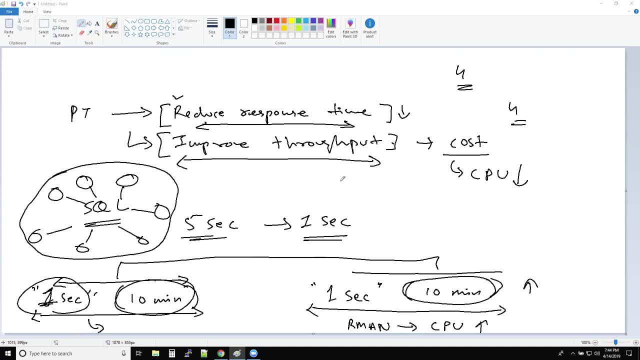